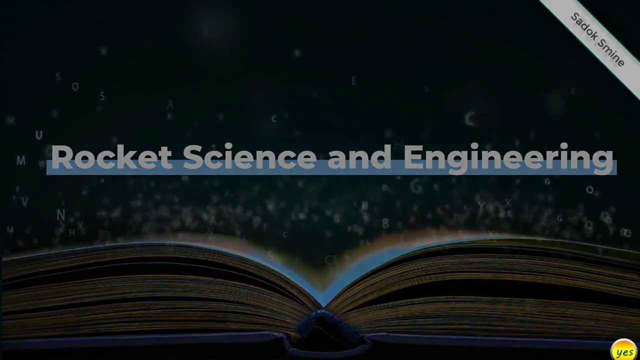 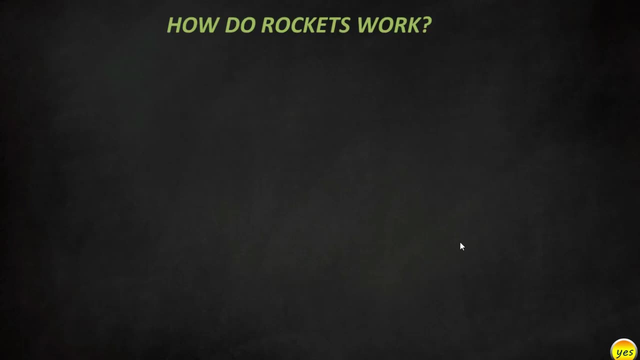 So in the previous video I've been talking about something, but never really explaining it, and that is thrust. So one might ask what is thrust? Well, to answer that, we have to ask ourselves: how do rockets work? Well, rockets are based on the third, on a simple law, which is Newton's third law of motion. 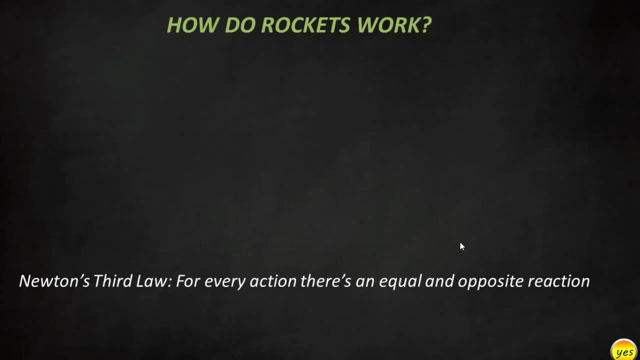 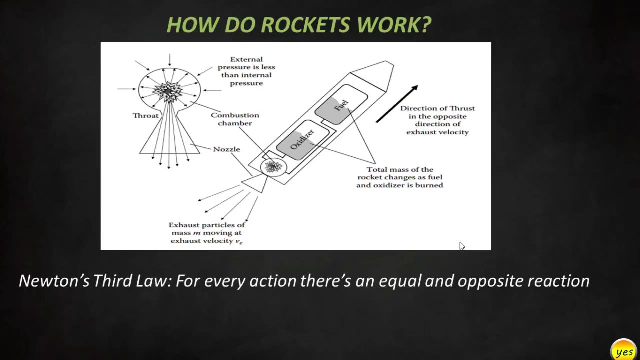 which states that for every action, that is an equal and opposite reaction. how does that apply to rockets? Well, as I said in the previous video, and if we consider a chemical rocket here, so we're going to- we're going to focus on chemical rockets and specifically, 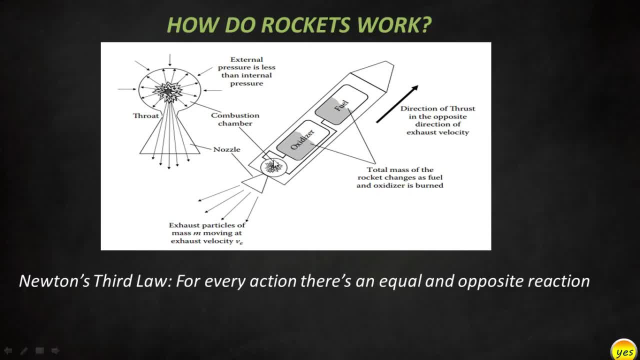 on liquid fuel rocket engines. So, as we said in the previous videos, fuel and oxidizers- and oxidizer are considered propellants. So these propellants will mix together inside the combustion chamber in here And, as you see, in here too, so they will mix together and then they get ignited. 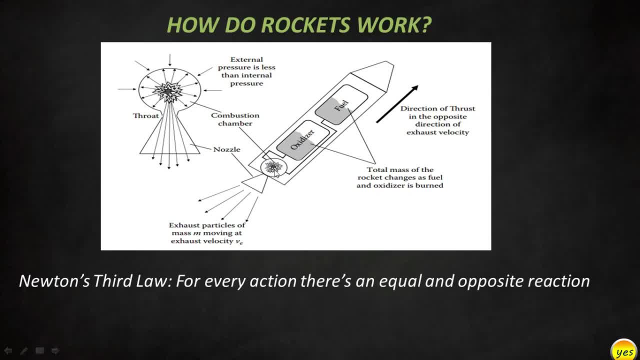 So they will burn And therefore, after they burn, they will get heated up. after heating them up Now, they will vaporize and we've got hot gases now inside that combustion chamber And due to that hot gases and due to that great amount of heat that was. 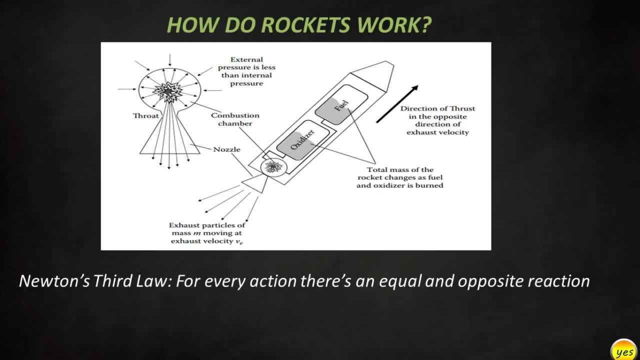 transferred due to the great amount of heat and the great temperature there, the high, the really high temperature there. Now we've got a high pressure And so these hot gases, Those hot gases inside the combustion chamber, will try to get out through that nozzle because the pressure or the ambient pressure, 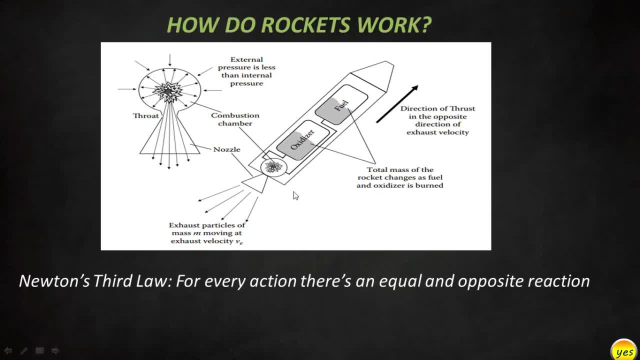 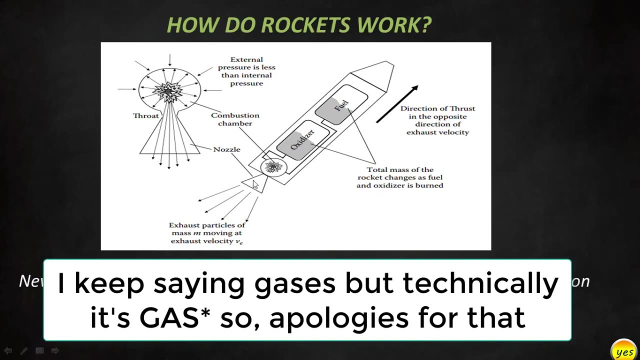 the atmospheric pressure surrounding that rocket is less than the pressure inside that combustion chamber, So the gases will try to get out. And now we're talking about exhaust gases. Now, once those exhaust gases leave the rocket or leave the nozzle, we're talking about an 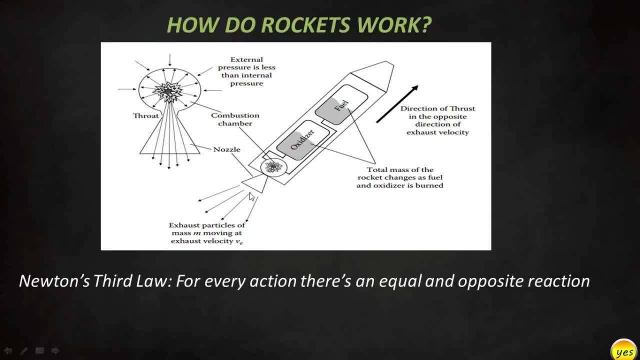 action here. So that is the action. The action is the gases being or getting out of that nozzle. So as they try to come out of that nozzle, as an action we will get a reaction, which is, of course, the lift up of the rocket.